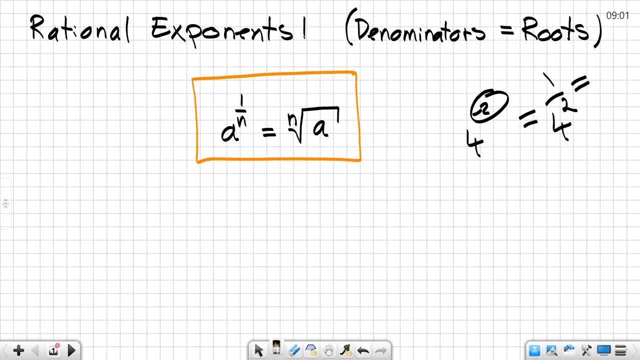 real quick. this means 1 over 4 to the positive second, so that would be 1 over 16.. But what happens if I put fractions up there in my exponents? Well, fractions, let's first look when I have a 1 up here, so only focus on this number down there, the denominator That. 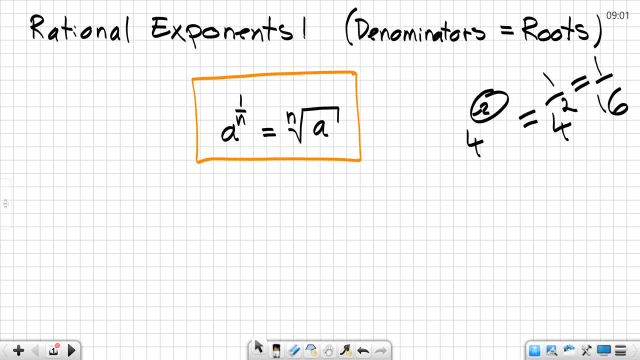 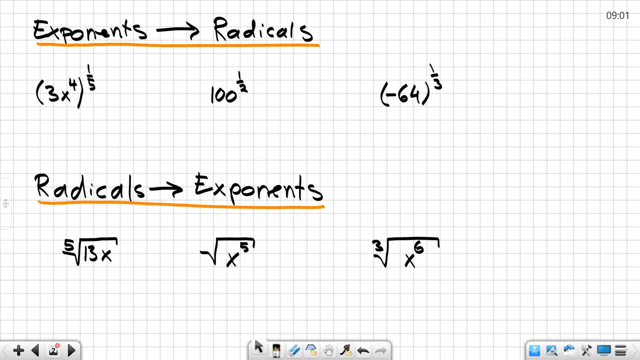 will just be the nth root out of a. So, in other words, the denominators are roots. Now, denominators mean roots. Let's do a few examples of this. Let's first try to rewrite from one expression to another. The first thing that we are trying to do is from: 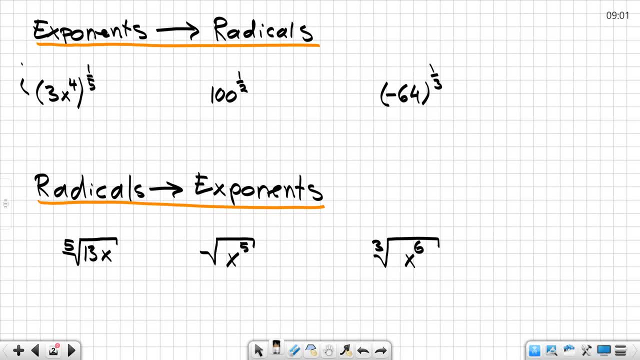 the exponent to a radical. Let's try to take something with an exponent and rewrite it with a radical sign. So the 3x to the 4th raised to the 1, 5th. If I want to rewrite this, this will be the exact same thing. The denominator is 5.. 5 down here is a 5. And 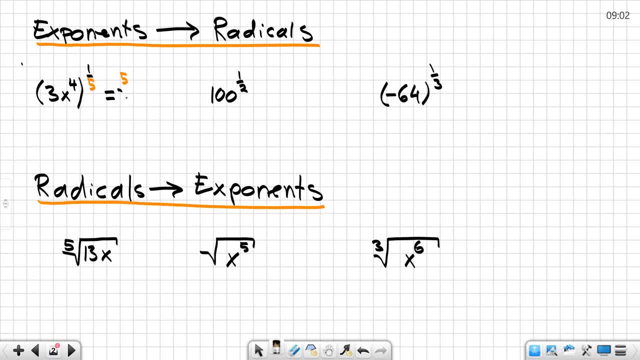 that means that I will just simply get the 5th root out of 3x to the 4th. This is the exact same thing. Both expressions are equivalent. It's just a different way to write this. So we are just practicing this at the moment. 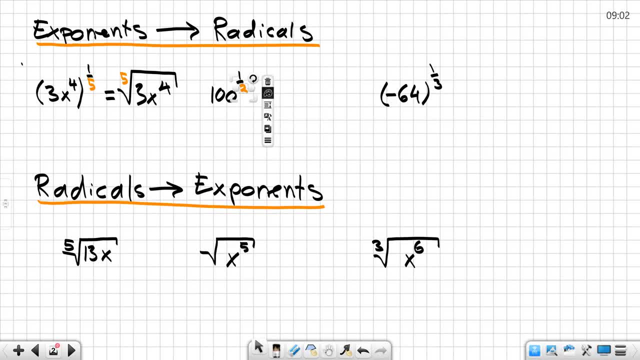 So 100 raised to the 1 half means nothing else but well, the square root out of 100.. We know that, strictly speaking, this 2 up here is not necessary to write. It can go away. We do not need to write this, You just need to understand that it is there And where. 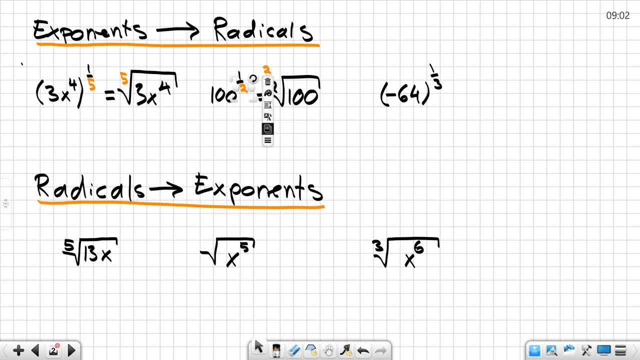 does it come from? It comes from this 2 right here. Well, let me throw that 2 up here. And what is this? Well, in this case, I can simplify this: The square root of 100 is nothing else but 10.. So, really quickly, what does 4 raised to the 1 half mean? Well, 4 raised. 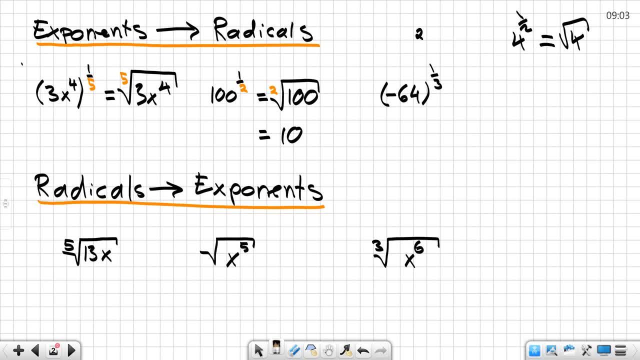 to the 1 half is going to be the square root of 4.. And that is equal to 2.. Let's have another example here that we have written down. This is the negative 64.. And this is the square root of 4 raised to the 1 third. What are we going to do? We are just 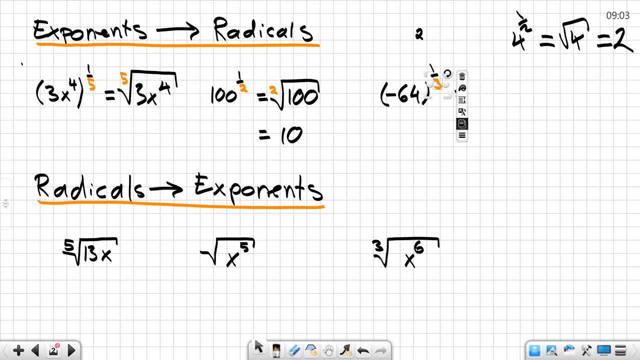 going to look at the denominator down here. I have a 3. And that means I will get, if I rewrite this, the third root, the cubic root, out of a negative 64. And the cubic root out of a negative 64,. if I rewrite it like this, maybe that will help, Because in 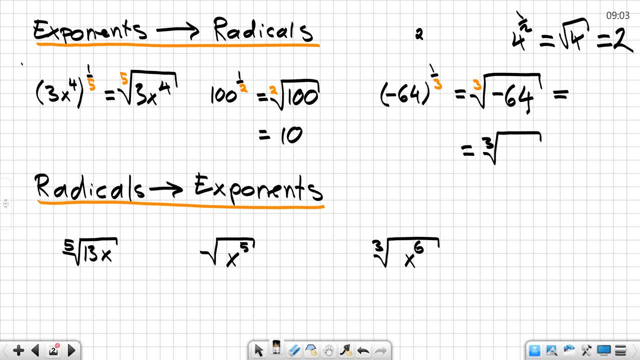 the future. this is what we are going to do. A negative 64 is the same thing as a negative 4 raised to the third power, And we have seen in the last lecture that this will be just negative 4.. All right, Now let's go in the other direction. Let's go and write something with a rational. 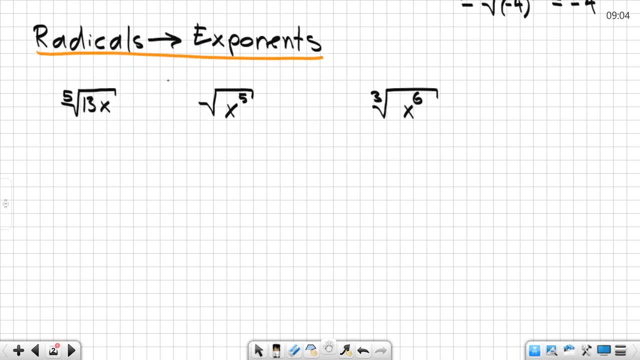 exponent that had a radical sign to begin with. So if I have here the fifth root out of 13x and I want to rewrite this, I want to take this and I want to rewrite this with a rational exponent, Then all what I have to do I take this radicand. 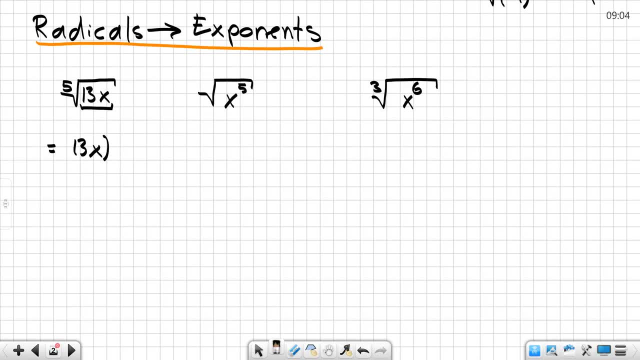 the 13x, and I have to be careful that I will place parentheses around this. Now I'm going to raise this to the 1- 5th. Remember the denominators are 1, 1, 1, 1, 1, 1.. That's the. 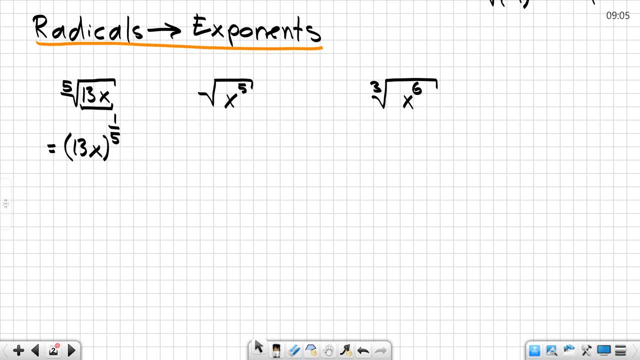 denominator: the radicals. those are the roots, and that was already. it. Doing the same thing with the next expression here. Well, what number is the index? in this case? This was a 2 that we don't need to write if I just write the square root, but I 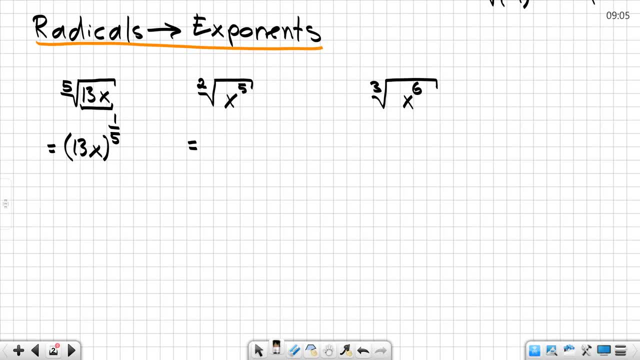 need to understand it, is there? So if I now rewrite this, I do the same thing as before. the radicand was x to the fifth and I raise this to the one half. So the square root is nothing else but something raised to the one half. But 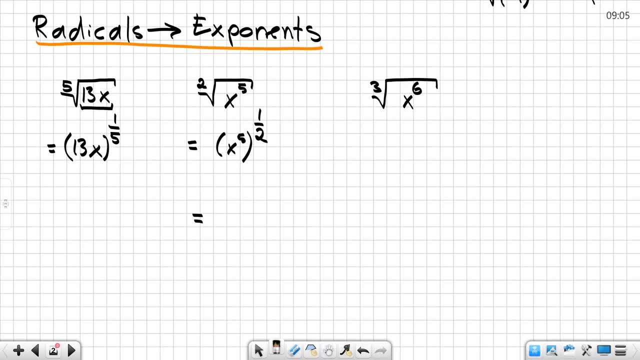 here's the thing. in this particular case, I can do something else. I have one exponent and raise it to another exponent. So what did my rule say I'm supposed to do with these two exponents? We have seen this in some sections before. At that moment, you will have to. 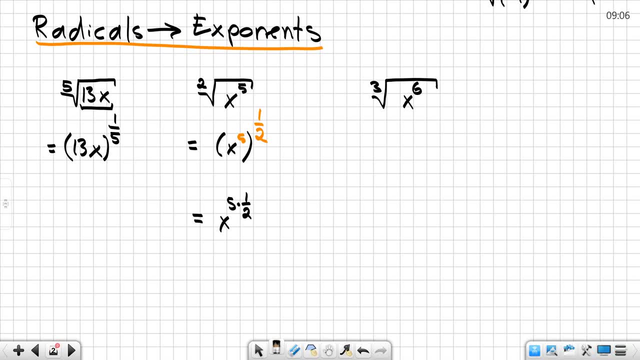 multiply your exponents And five times one half, that is nothing else but x raised to the 5 over 2.. And these are the ones that we will be looking at more in the near future. So if I do this, the same thing with the next expression: 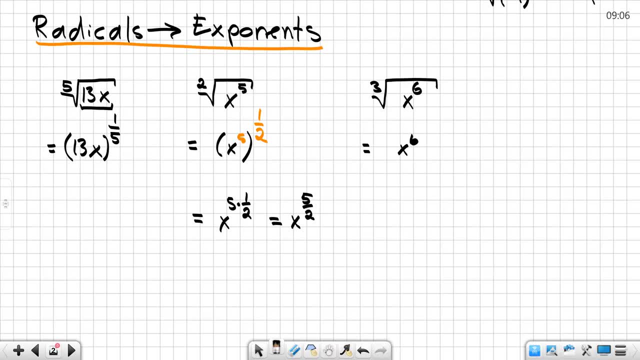 right here I have x to the sixth, which was the radicand, and I raise this to the one-third. Why do I raise it to the one-third? Because this was the cubic root and roots are numbers from the denominator, And now I see that I have. 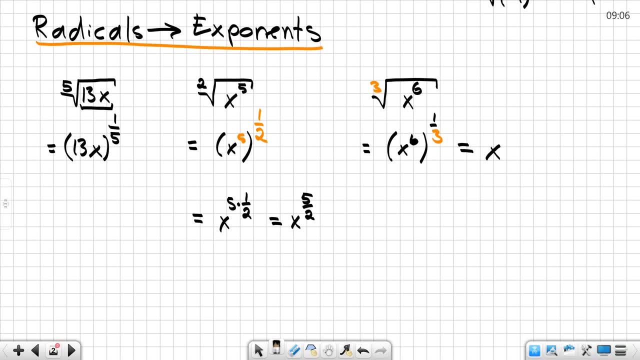 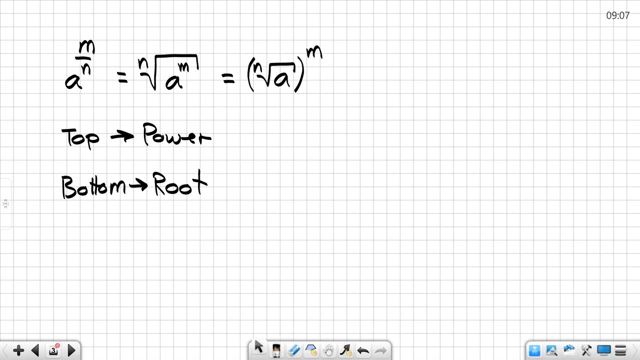 one exponent raised to another exponent. So I will have to multiply these two exponents, And six times one-thirds that will be: 6 divided by 3 is nothing else but x squared. So we are now starting to make it more complicated, Slowly but steady. If 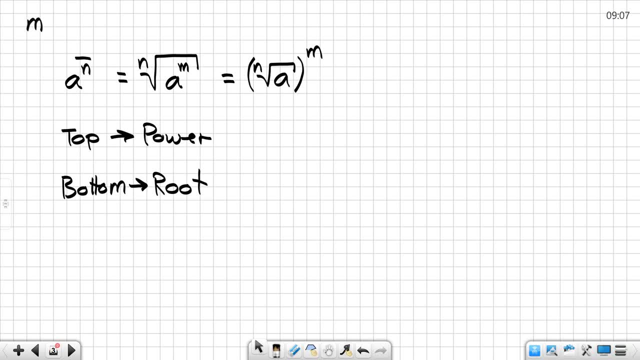 I not just have one up here in my exponent, in my numerator, but some number m, Then this will be the same thing, as The bottom stays the same. The bottom in your exc, in your exponent is the root, But the top is the power. So in other words you 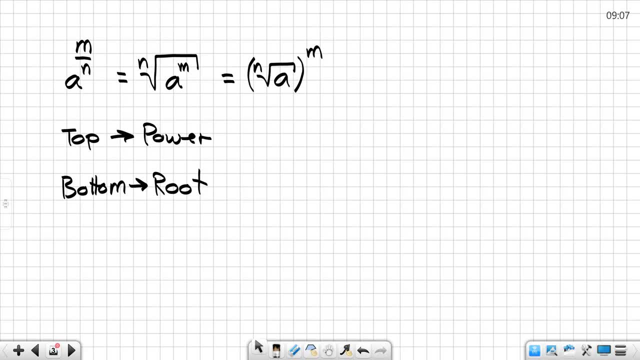 can think about it like this. I'm allowed to write this in two different ways. First, take something and raise it to the and m power, And then take the n through out of it from inside to outside. take the nth root and then raise it to the m power. If you go backwards, just do. 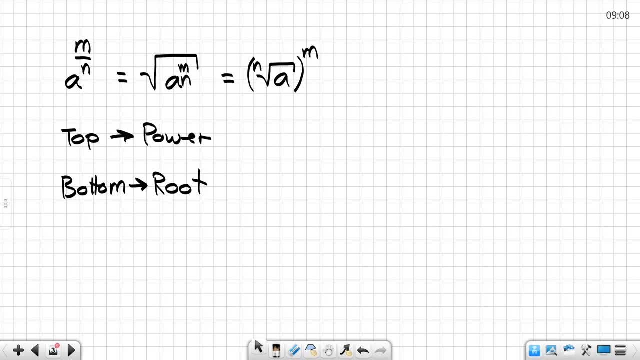 this, This outside here just goes underneath the m. if you want to rewrite it. You see that This n on the outside just goes underneath the m, if you want to rewrite this Again. the bottom is the root, the top is the power. I have not. 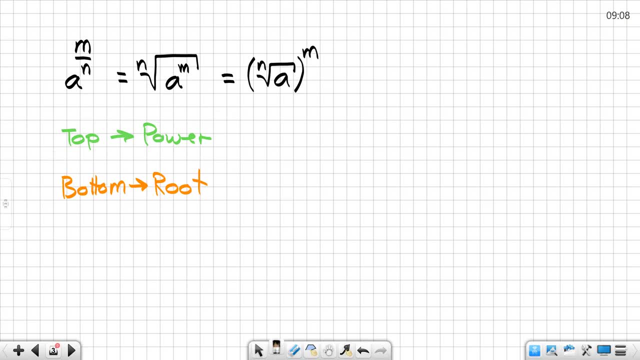 chosen wisely. Oh, I did. Sometimes I like to remind myself by drawing a little picture. All right, let's try to do this. Well, what do we have here? This is supposed to be a tree, and where on the tree are usually your roots On the bottom? I hope that helps. All right, so? 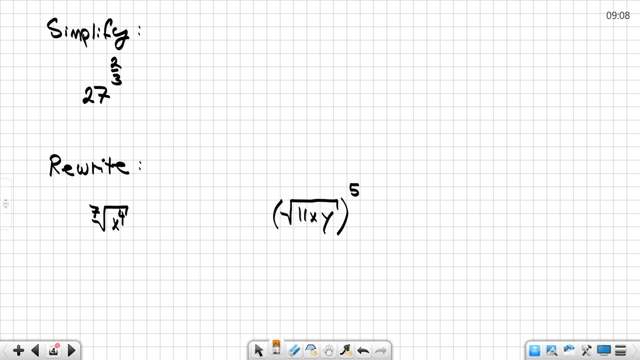 let's go ahead and simplify some things: 27 raised to the 2, 3rd power. So what I will do? I will rewrite this. There is a 3 in the denominator right here and that will turn into a cubic root of 27.. And there is a 2 in the 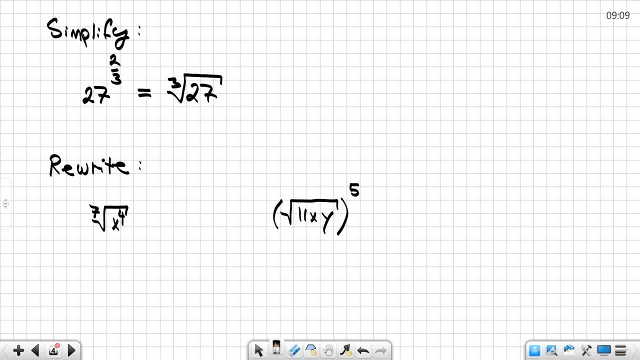 numerator and that will turn this into an exponential. Now, where I put the exponent doesn't really matter. if I would put it in here, That would make my life a little bit more difficult, But I'm going to put it on the outside. And why did I put this on the outside? Because now I see that the cubic 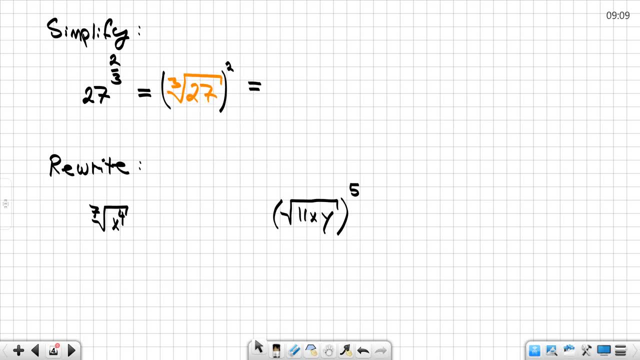 root out of 27.. Oh my goodness, That was actually something nice. That was something easy. I know what the cubic root out of 27 is, and that is 3.. So that's 3.. 3 raised to the 3rd power is 27.. 27 is a cubic number. Now I just have to look. 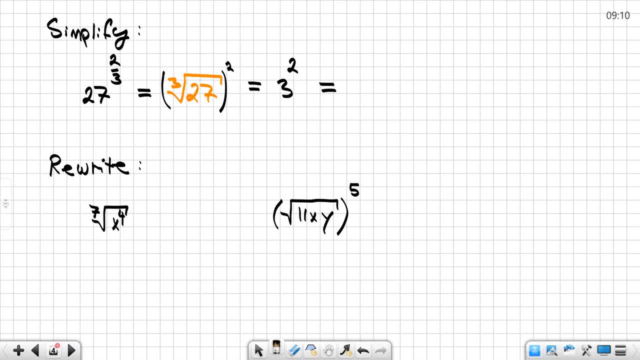 at the 2 as an exponent on the outside, and 3 raised to the 2nd power, That will give me 9.. So, in other words, 27 raised to the 2- 3rds is nothing else but your number 9.. Let's. 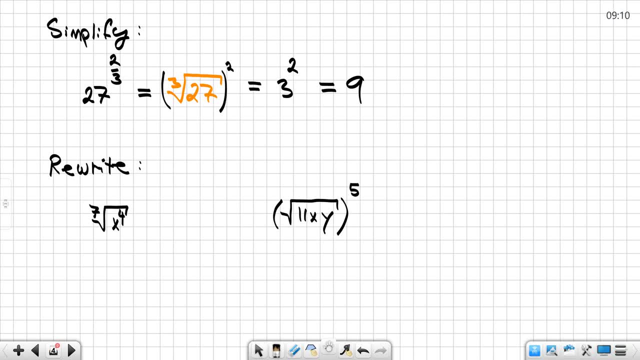 rewrite some things: The 7th root out of x, raised to the 4th power. We have technically done an example like this already before, But let's do it again. This means nothing else but this: This is x to the 4th, and raise this to the 1- 7th, And if I multiply now the 4 and the 1- 7th, I get x. 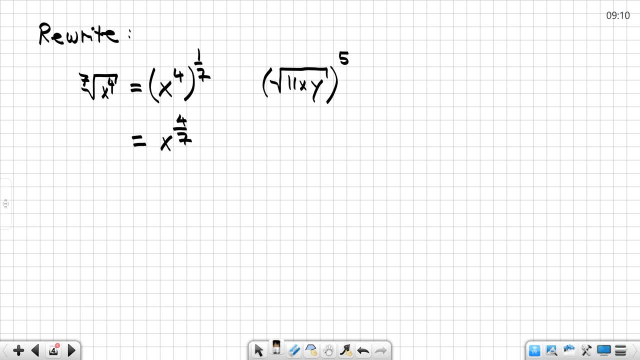 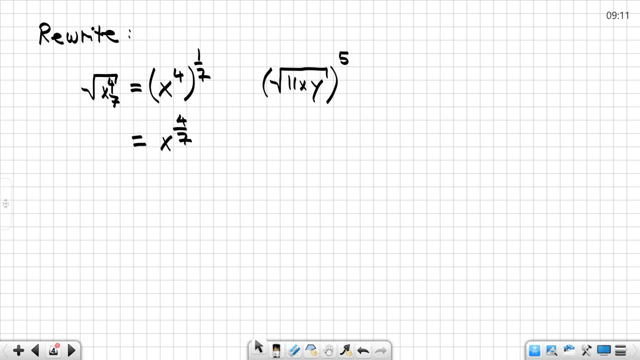 this 7 right here goes in the bottom of your exponent, And you see that this is exactly what happened right here. 4 over 7 is what we will end up with, But you need to know how you got there. So I'm going to do the same thing with this one here on the right. 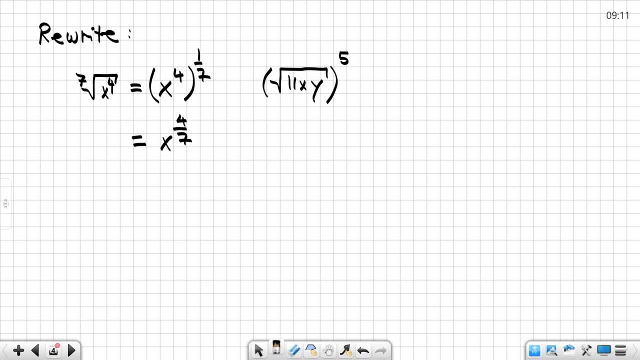 hand side. Now what do we have? We have the square root of x raised to the 4th power. We have the square root of 11, x, y raised to the 5th power. So if I want to rewrite this, 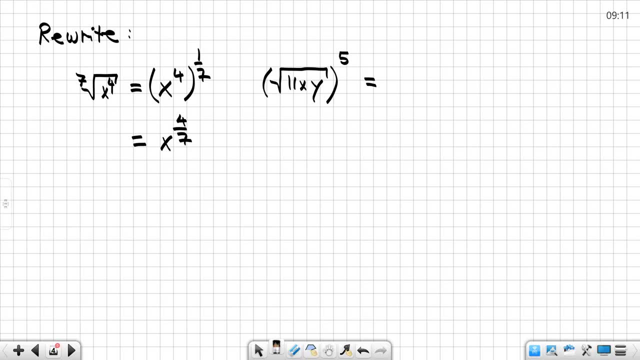 then what I will have to do. I look on the inside of the parentheses and that will give me now 11 x times y. This was the square root. So this 2 right here goes under the 5.. The 5 stays on the top And I get 5 over 2.. The long way to see why this works this. 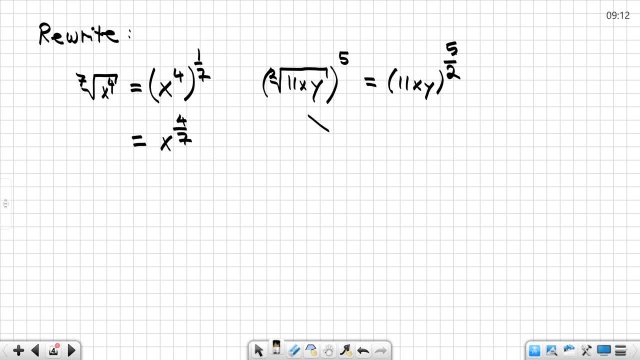 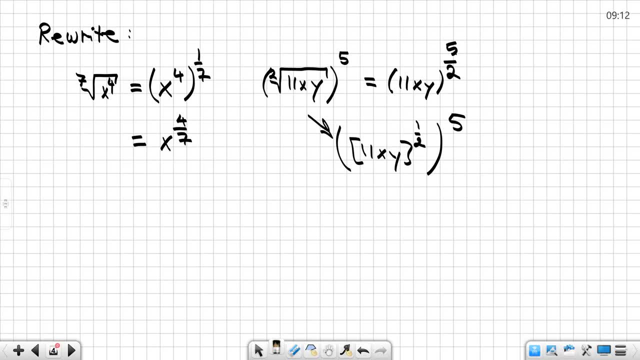 then I still had 11 x- y raised to the 5th power on the outside. So I first just rewrote the radical And now I have to multiply the two exponents And I will get 11 x- y raised to the 5 over 2, which is exactly what we got right here. All right, So now we are going. 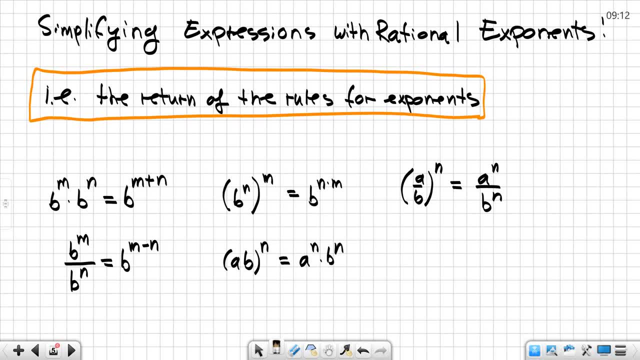 to look at how to simplify expressions with rational exponents. And yes, it's the return of the rules for exponents. All of the rules are exactly the same. The rules never change. The rules all stay exactly the same. These are the rules that we have already seen for. 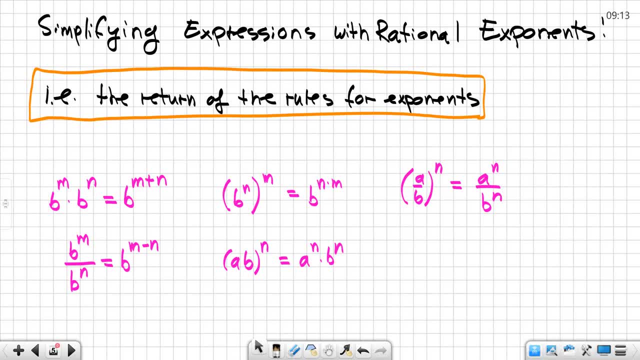 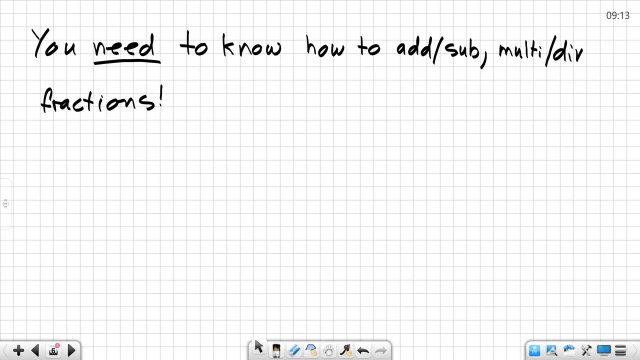 exponents. Let's make them pink so that they are staying out for us, All of those rules we are using now. But remember, the exponents now will be fractions for us. So the moral of the story is You need to know how to add, subtract, multiply and divide fractions. If you need a reminder, 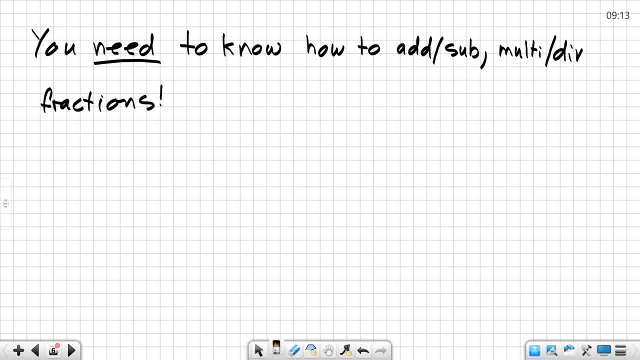 on this. go back and look it up. You need to know how to do these Adding and subtraction. you need to have the same denominator. If you don't have it yet in the beginning, then you need to manipulate them. Multiplication is simple: You just multiply and divide You. 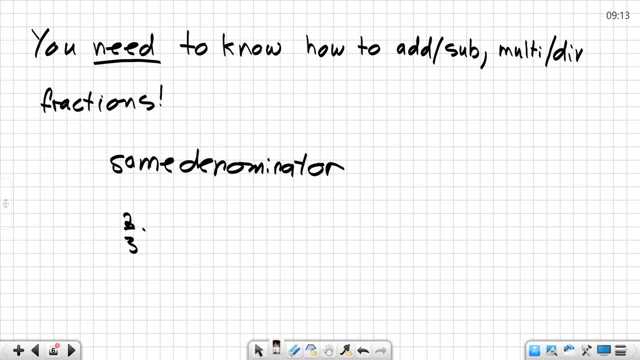 just multiply straight across, For instance, 2 over 3 multiplied with 5 over 8.. You just multiply this strictly speaking straight across: 2 times 5, divided by 3 times 8.. And then you simplify Really quickly. what did I do with division? What did I have there? 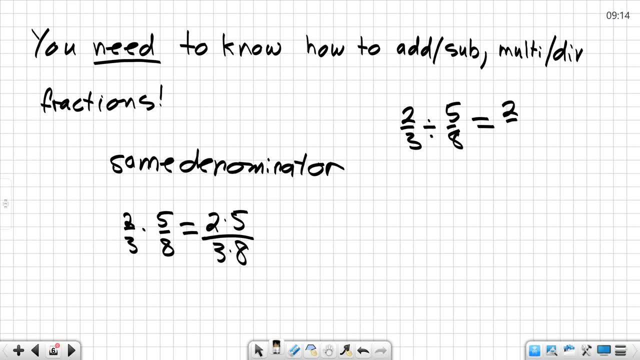 5 over 8.. Division: you multiply with the reciprocal With 5 over 8.. And then you do the same thing as division: You multiply with the reciprocal. You multiply with the reciprocal before, two times five divided by three times eight. all right, that was a really, really really. 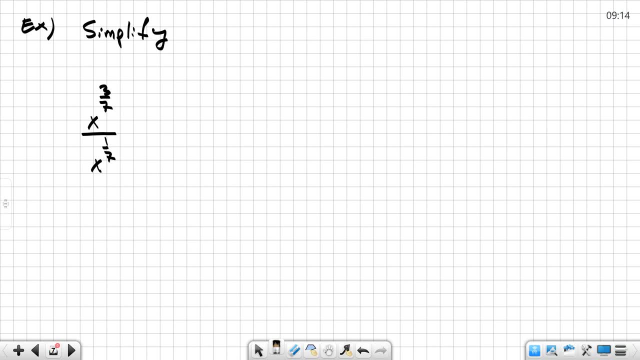 quick reminder. so if i want to simplify now, x raised to the three over seven divided by x raised to the one over seven, what did my rule say? top minus bottom, top minus bottom. the top exponent was three over seven. the bottom exponent is one over seven. now this is really nice because 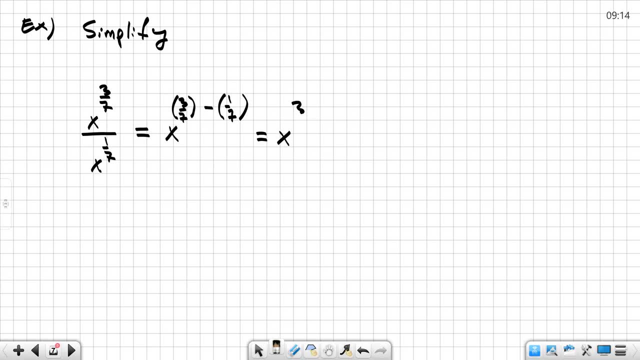 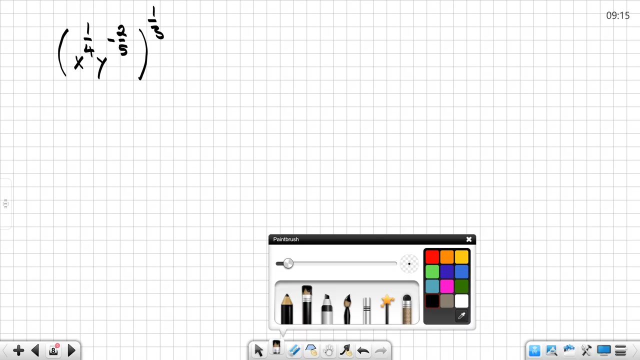 the denominators in both cases are the same, so i will get three minus one over seven, which is just two over seven. see, the only thing that was difficult here is how to subtract the denominators. all right, getting crazier you. we have to do several steps here. what was the rule that we had when we had an exponent on the? 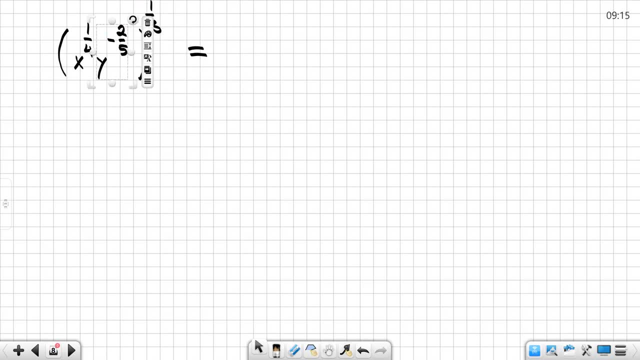 outside of something that was multiplied that right here jumps to both. let me write it down in detail so that you see exactly what is happening: x raised to the one. fourth raised that to the one third times. y raised to the negative. two-fifth raised that one as well to the one-third. so both factors are. 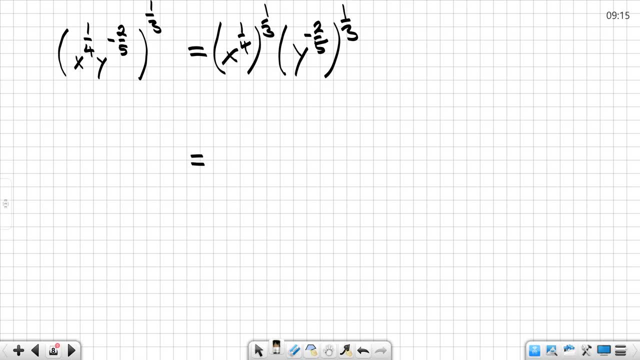 being raised to the one-third. now my rule said for this that i had to multiply the exponent. i have a negative two-fifths and i multiply it with one-thirds and what i get when i multiply these fractions out, i get a negative two-fifths of the one-third, which appears to be a negative one-third. i give it aboarater at eating a qugia, which is a quagmendium. so we're and and we use our hands to separate the critube, which is a torchout, between these two items, which is the expression that weren't part of the expression. and octopus, you ring the bell and the arrow to the color income, which is what we're looking at right now. so, as i, we'll just go on to the method by putting that find the effect. 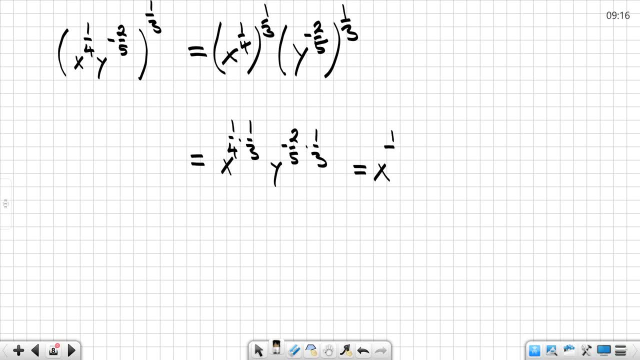 fractions out, i get 1 4th times 1. 3rd is 1 over 12. y raised to the negative, 2 5th times 1. 3rd, that is a negative 2 over 15. remember when we have negative exponents, negative exponents. 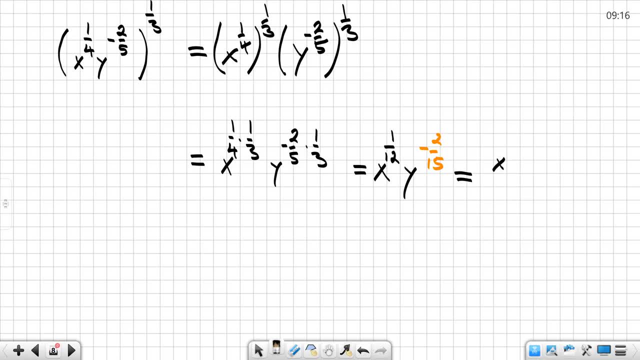 will be turned into positive exponents by simply changing their position. it drops into the denominator and i am done, let's do one. that looks really crazy: 5 raised to the 3, 4th times 5 raised to the 1 half, and i believe that this 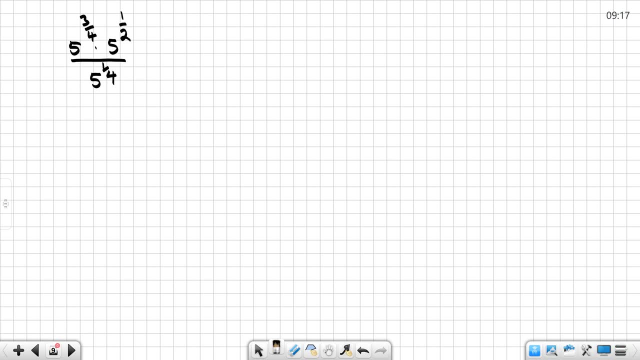 should be our last, except now. there will be one more example after this, so let's just do it one step after another. i look at the top first. so what rule do i have? at the top we are supposed to add the, the exponents. so what in the world is 3 4th plus 1 half? well, they do not have the same denominator, but the. 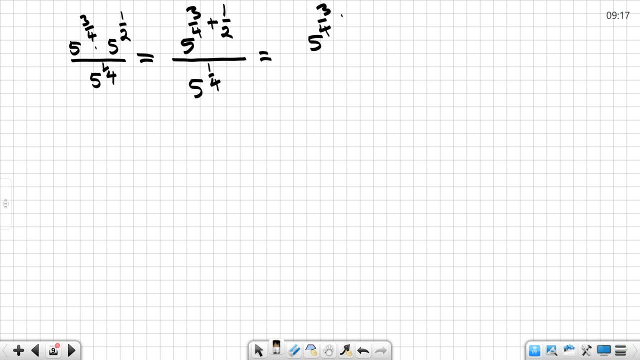 least common denominator is 4, so i take 1: half and i multiply the top and the bottom by 2 to get 2 over 4, and now plus 3 over 4, plus 2 over 4, well, that is going to be 5 over 4. 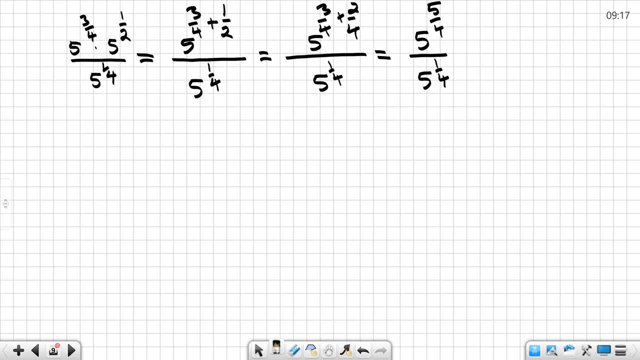 so, in short, 3 4th plus 1 half is 5 over 4. this is supposed to be a 4, all right. last step: top minus bottom, 5 over 4 minus 1 over 4. let's have a look what is 5 over 4 minus 1 over 4, that is, 5 minus 1. 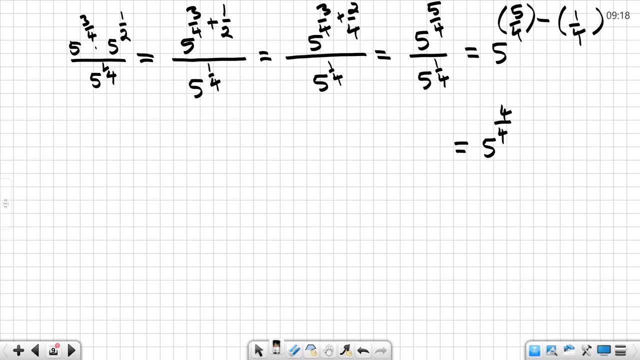 which is 4 over 4. well, and 4 over 4 is nothing else but 1, and 5 raised to the 1 is just 5. so this is kind of like a mathematical joke that this whole thing turns out to be exactly equal to 5. 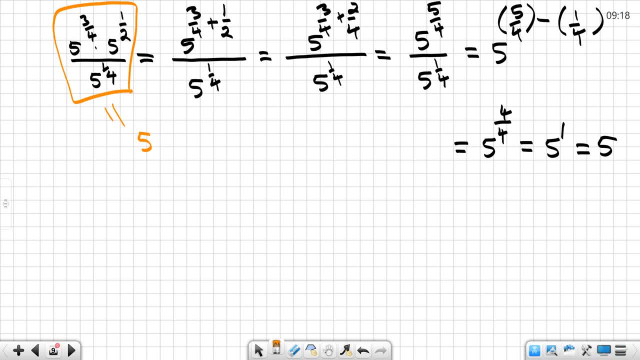 after doing all of our simplifications. last example for today: 50x to the 1 3rd divided by 10x to the 4 3rd. so we are splitting this into two problems. this is 50x to the 1 3rd and this is 50x to the 1: 3rd.